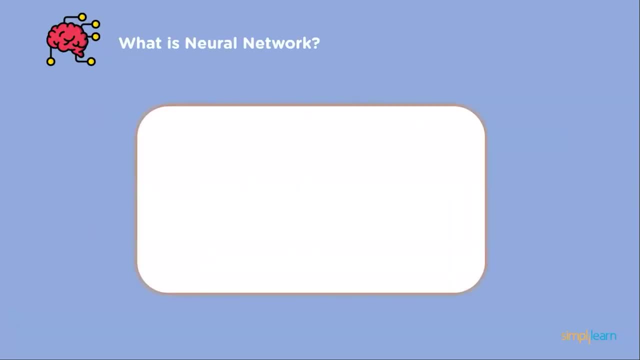 ado, let's begin. What is neural network? In simple terms, an artificial neural network can be called as a system of hardware and software that is framed after how neurons in the human brain function. Artificial neural networks are the other name for neural networks. Our brain has billions of. 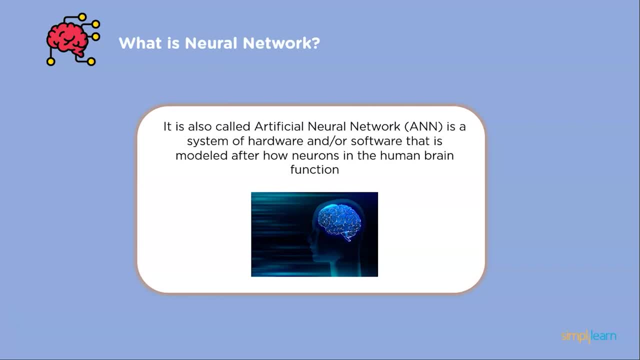 neurons. They are all interconnected. Neural networks contains three major layers. They are an input layer, an output layer and a hidden layer. Let us define neural networks first. An artificial intelligence technique called a neural network instructs computers to analyze data in a manner modeled after the human brain. Deep learning is a sort of machine learning. 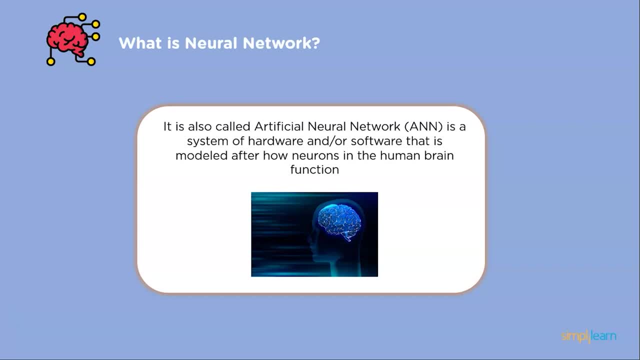 that employs interconnected neurons or nodes in a layered framework to mimic the human brain Functions, like that of the human brain In a neural network. a neuron is a mathematical function that gathers and categorizes data following a particular architecture. The network is similar to statistical techniques like regression analysis and curve fitting. So 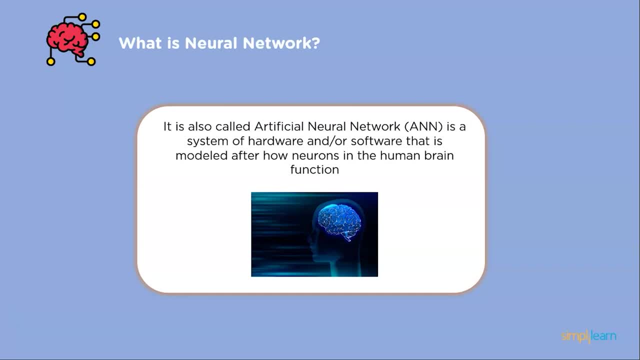 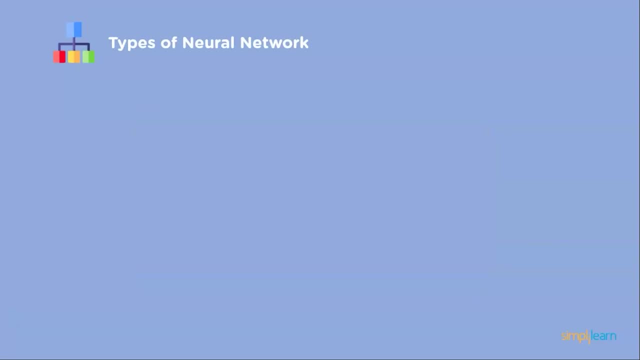 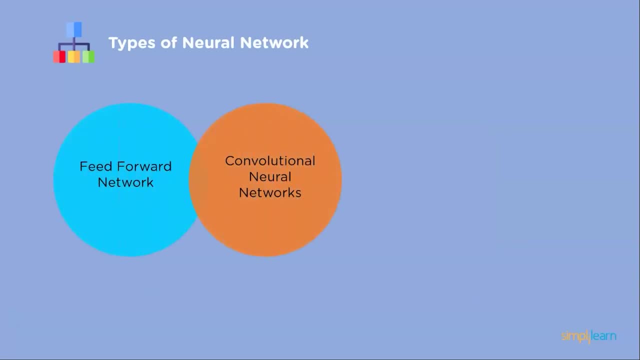 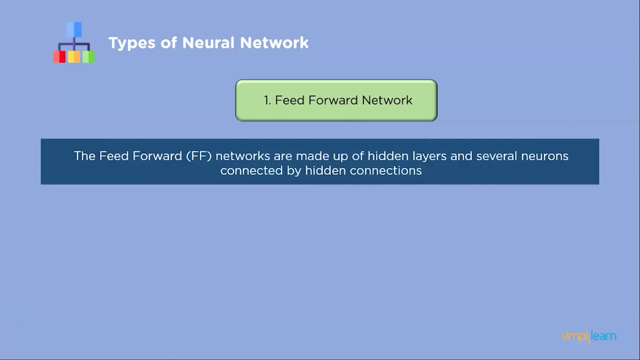 understand feedforward network Up next, convolutional neural network, recurrent neural network and finally, multilayer perception. First we will understand feedforward network. The feedforward networks are made up of hidden layers and several neurons connected by hidden connections. 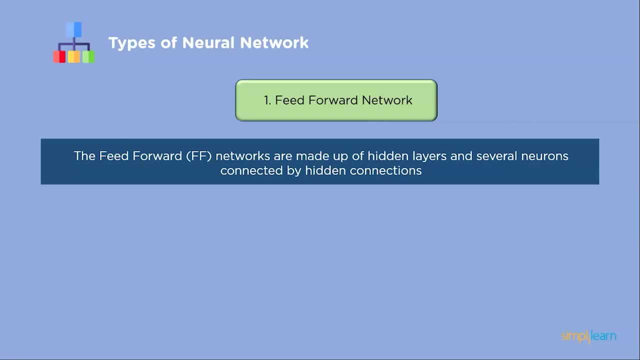 Since there is no backward propagation and the data only travels in one direction, these are referred to as feedforward systems. Convolution neural network. It is a neural network for deep learning which learns directly from given data. It is used to recognize the given patterns, objects and faces. Convolution- 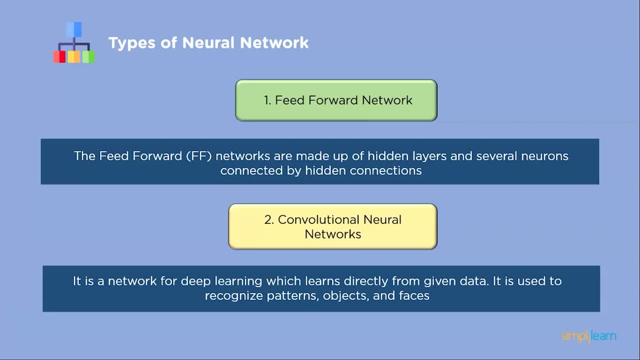 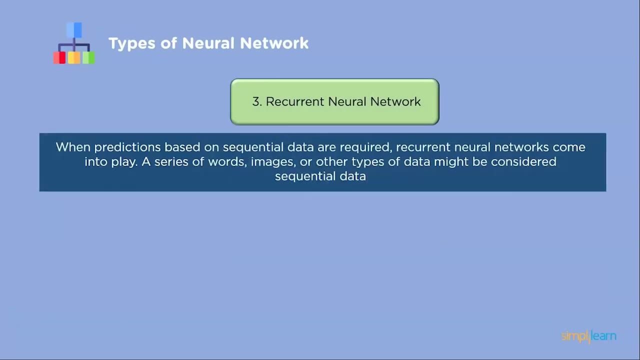 neural networks are the most popular for image classification. Multiple convolutional layers of CNN are in charge of extracting significant features from the image. Next we will understand recurrent neural network. When predictions based on sequential data are required, the recurrent neural networks comes into play. A series of words, images, 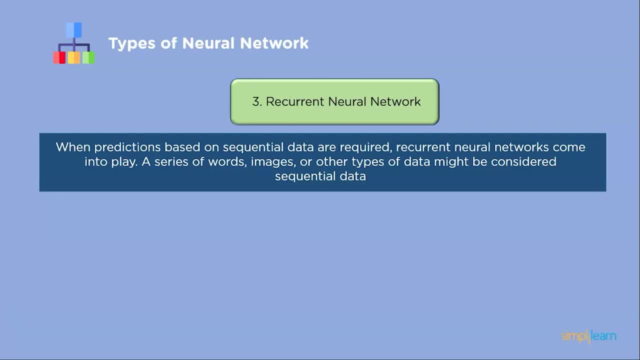 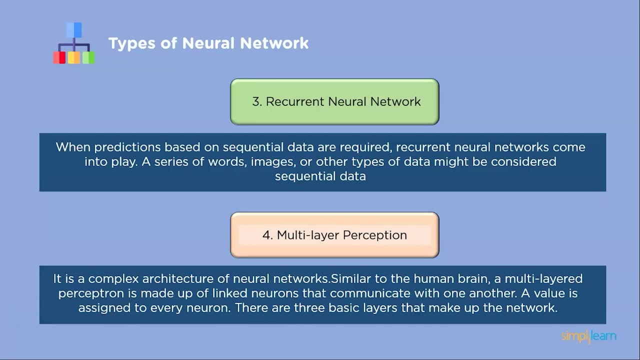 or other data types might be called sequential Multilayer perception. It is a complex architecture of neural networks. Like the human brain, a multilayer perceptron is made up of linked neurons communicating with another, Because the atoms communicate with proteins and the 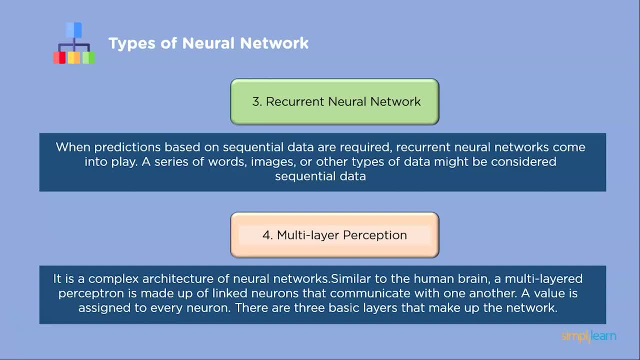 neutrons communicate with fibers. it makes the neurons atheistic When material roasts a value is assigned to every neuron. three basic layers make up the network. perceptrons with numerous hidden layers and activation mechanisms are known as multi-layer perceptrons gradient. 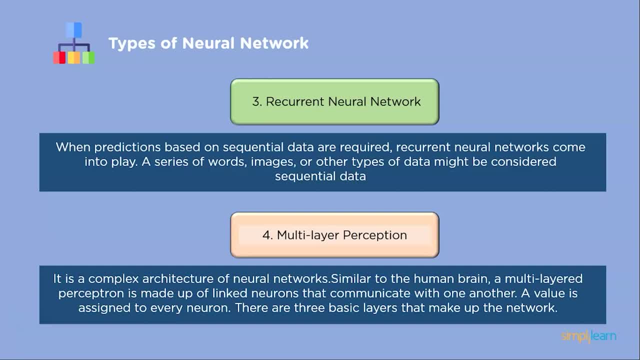 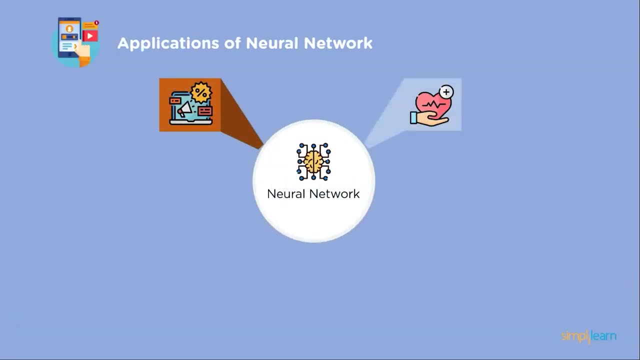 descent is used to update the weights during the learning process, which is conducted under supervision. these are all the important types of neural networks. now we will see real world application of neural network. first we will cover about medical care, then comes sales and marketing up. next we will understand role of neural networks in personal assistance. 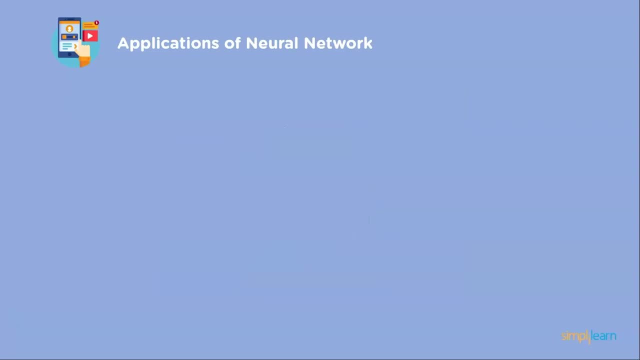 and last but important application is social media role of neural network in medical care. oncology uses artificial neural networks to train algorithms that can detect malignant tissues at the microscopic level with the same accuracy as skilled medical professionals. using facial analysis on the images of the patients, certain rare diseases that can appear physically can be detected in their earlier stages. therefore, 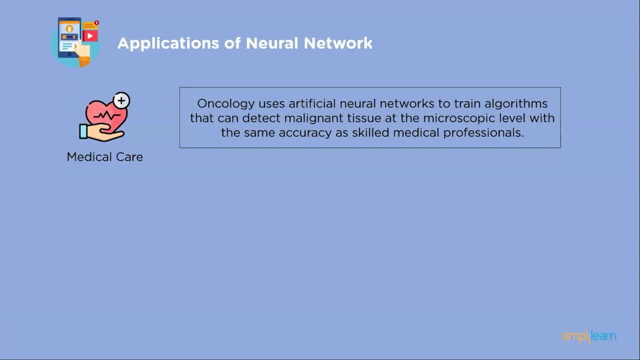 the widespread adoption of artificial neural networks in healthcare can only increase the diagnostic skills of healthcare professionals and, in the long run, the standard of health care globally. coming to sales and marketing, based on your previous browsing history, e-commerce sites like amazon and flipkart suggest that when you log in- similar to how zomato, swiggy, etc. 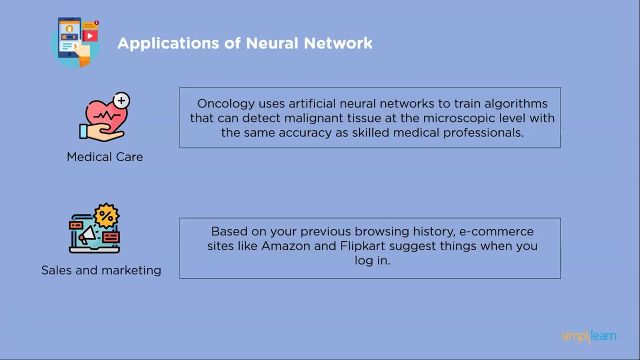 will present restaurants suggestions based on your preferences and previous order history. if you love pasta, it is done using individualized marketing, which is true across all your marketing categories, including book sites, movie services, hospitality sites, etc. so the technology behind all this is artificial neural networks. up next we will understand.